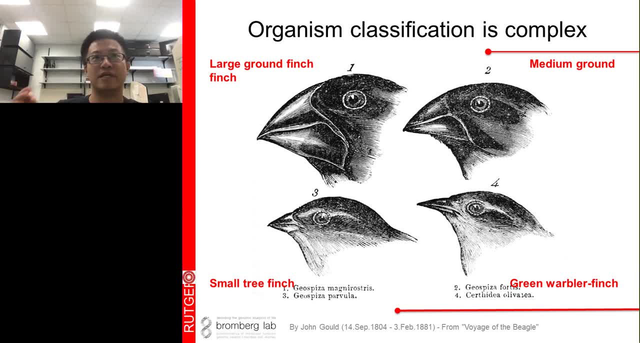 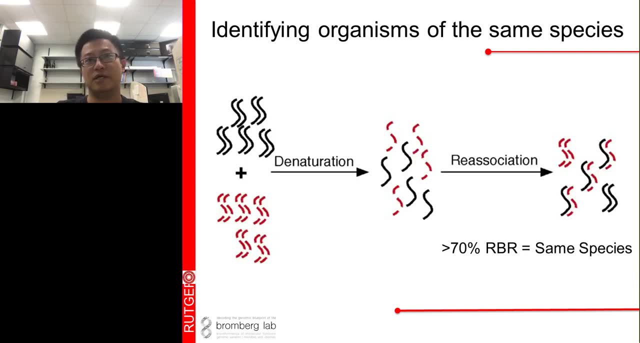 those tiny little bugs. we can't even see them, So this issue becomes even more complex. So currently, the gold standard to tell whether two bacteria of the same species or not is using this technique, which is called DNA-DNA hybridization. 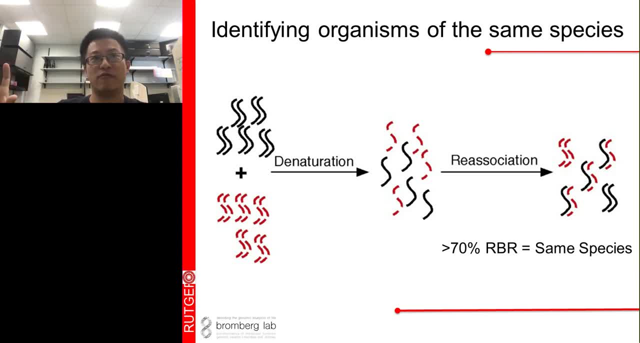 So the idea is that you take the DNA from both bacteria, you denature them into a single strand and then mix them together and let them re-associate, And then you count the rate of how much of this heterostranded DNA are there. 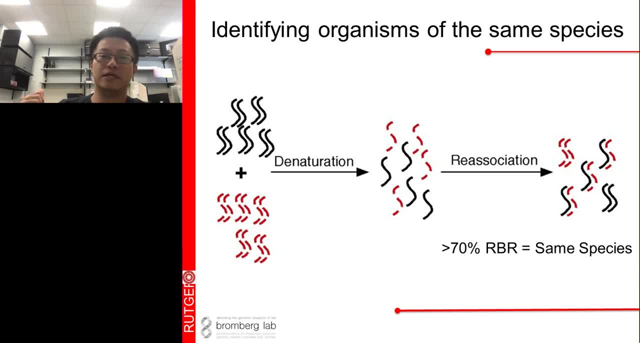 what is the fraction of those And the current? the current rule of thumb is that if there are more than 70%, then you can safely say that these two bacteria of the same species. But, however, although this technique is very accurate, but it's experimentally very demanding. 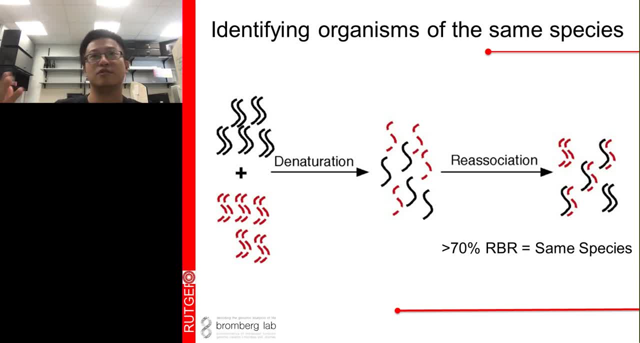 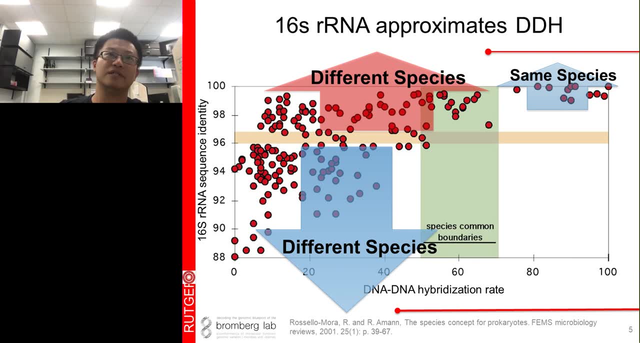 So it is challenging that people start to seek for another marker which is easier to use, And the answer that we have found is 16S-RNA. If you have been into this field, you must have heard about this gene, And it's always associated with a magical number. 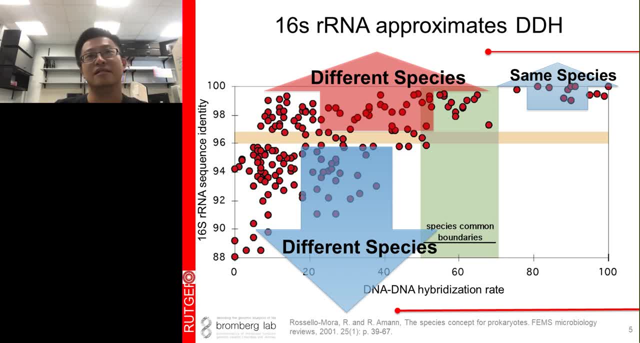 which is 97% sequence identity. So the rule of thumb is that if two bacteria share more than 97% sequence identity of their 16S-RNA, then they are of the same species. It is quite widely known and practically used in this field. 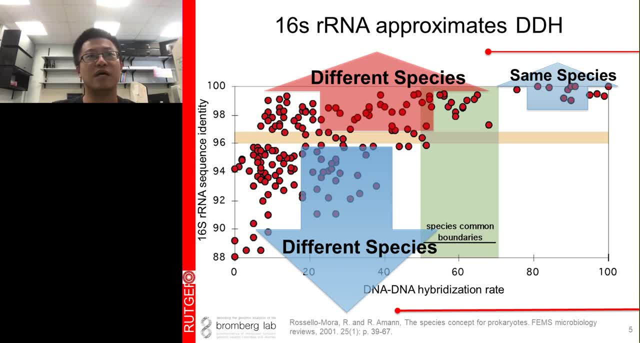 However, it's just not correct. So what do I mean here? So if you look at this picture, the X axis is this DNA hybridization rate and the Y axis is a 16S-RNA sequence identity, And each dot in this figure is a pair of organisms. 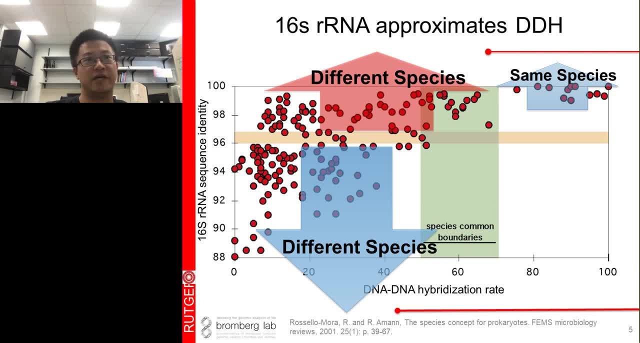 So if we look at all the organism pairs have less than 97% 16S-RNA sequence identity. we can see that. you know, without an exception, all of them belong to different species. But, however, if we look at above 97%, 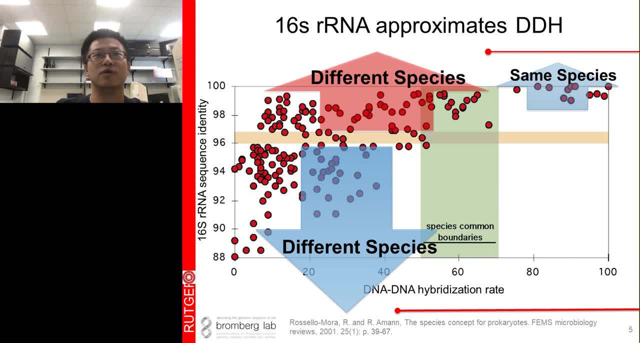 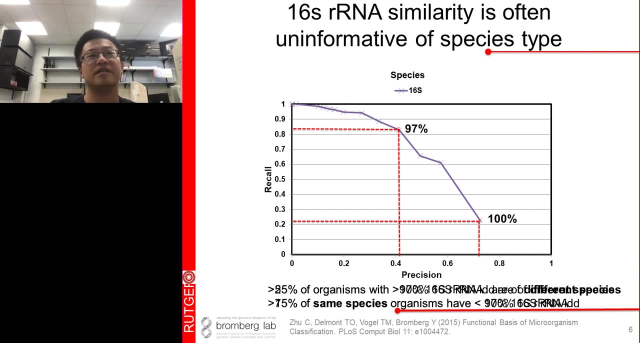 we both have the same species organism pairs as well as different species organism pairs, So this rule of thumb is not really accurate in reality. So in order to quantify, okay, how accurate it is really, so here is something that we did. So we collected 1,400 bacterial genomes from NCBI. 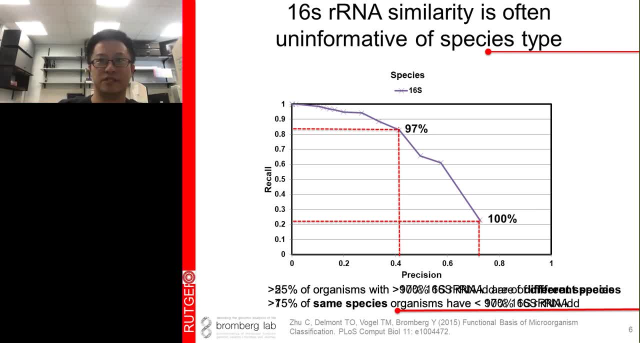 which covers the main, which covers the main, which covers the main domain of bacteria. And then I compared the 16S sequence identity across every single pair of these organisms and use that to predict whether these two organisms of the same species or not. 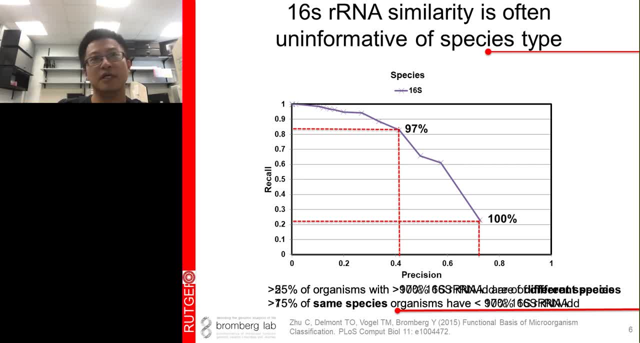 and the matter of the performance based on different cutoff. I choose So. for example, if we use this magic number of 97%, so for organism pairs that share more than 97% identity, there are more than 55% of organisms actually of different species. 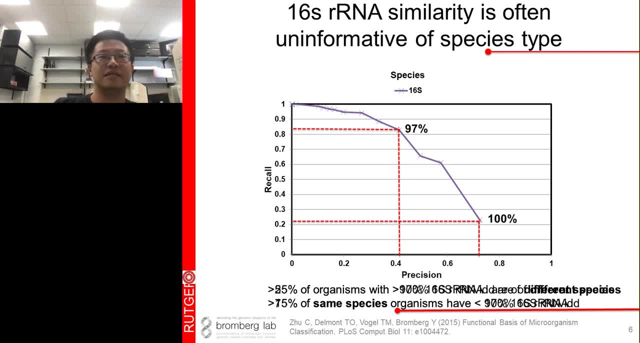 And then for those have less than 97% identity, actually more than 15% of them are of the same species. So what this says basically is that if you're using that famous rule of thumb to identify two bacteria to belong to the same species, using more than 97%, 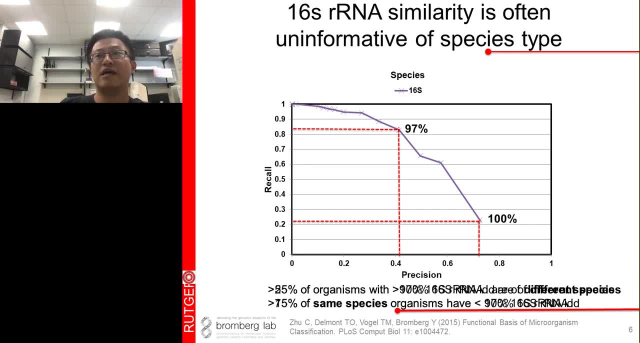 of 16S RNA identity, then you are more than 100% of them. So that's a lot of information. So that's a lot of information, So that's a lot of information, And then half of the time we'll make a mistake. 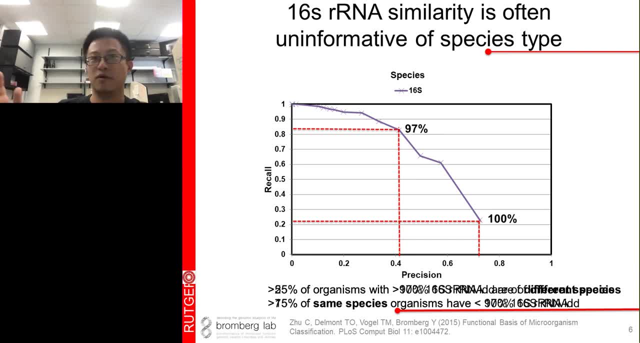 So people started to know this and then proposed that, okay, 97% is not stringent enough, Let's do 98%, 99%. So, but in reality here, even if we use 100%, just completely identical 16S RNA sequence. 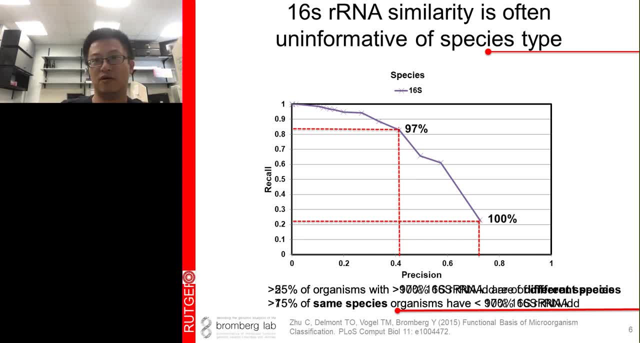 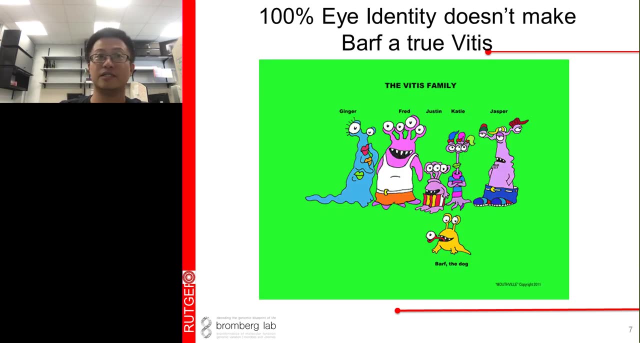 it still does not guarantee the two organism of the same species. The precision is actually just about 75%, like three out of four are correct. So by now I hope that I have convinced you that 16S RNA is not the best tool to use. 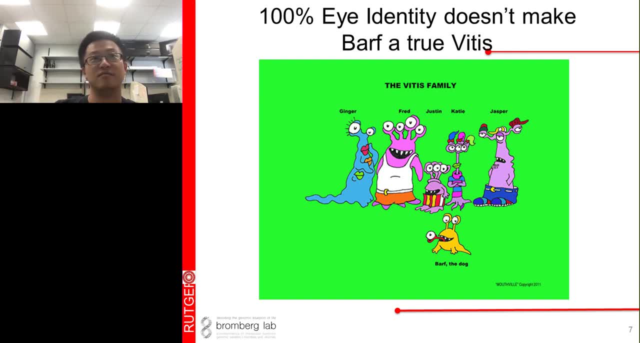 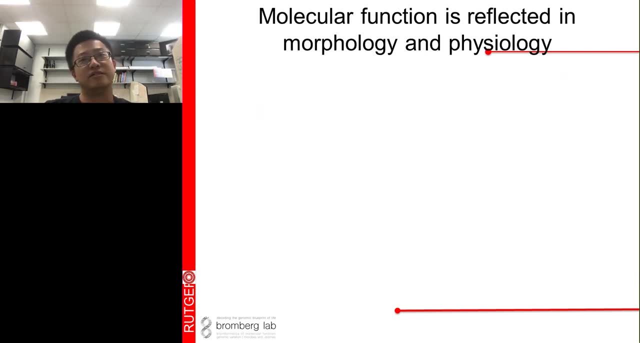 to identify same species, And this is just example. the 100% eye identity doesn't really make both a true virus. So if we cannot use 16S RNA, then what can we use instead, So we could actually measure all of the different features of a certain bacteria? 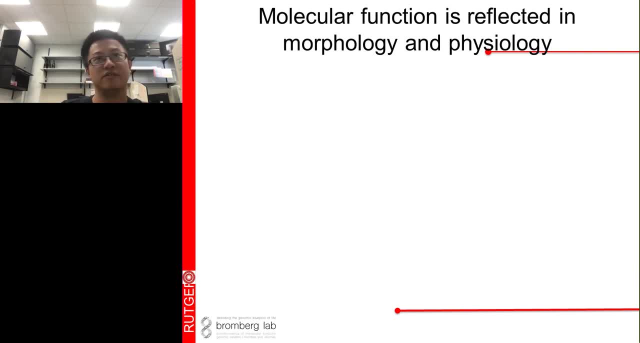 for example, like its morphology, physiology, through all those biochemical tests, and then just to find out all the details of what a bacterium is like, and then you can comparing that to the other bacteria and see if they are the same species. 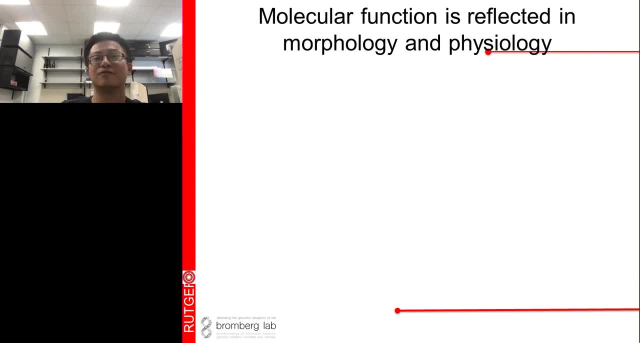 However, as just you can tell from my description, it requires a lot of work and it's almost impossible to measure everything. So is there a shortcut? So the shortcut is to measure everything. So the shortcut is to measure everything. The shortcut lies in the molecular function. 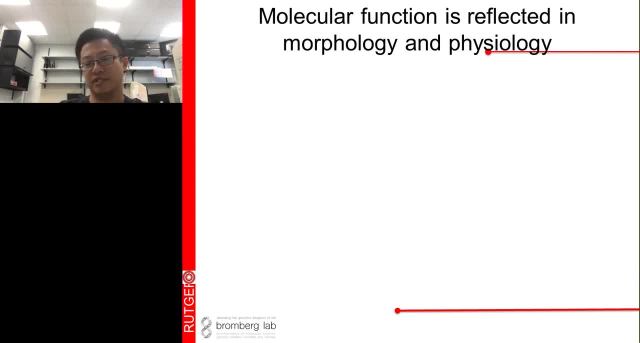 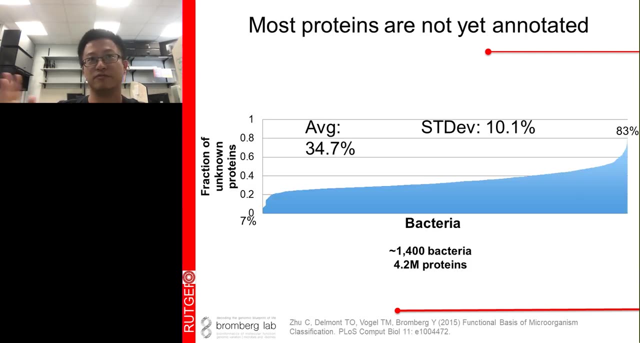 which is encoded in the organism, genomes, which reflects the morphology and the physiology of that bacteria. So if we were to use this function, molecular function, as a measure, then there are also some issues with it. The first thing is that a lot of the proteins- 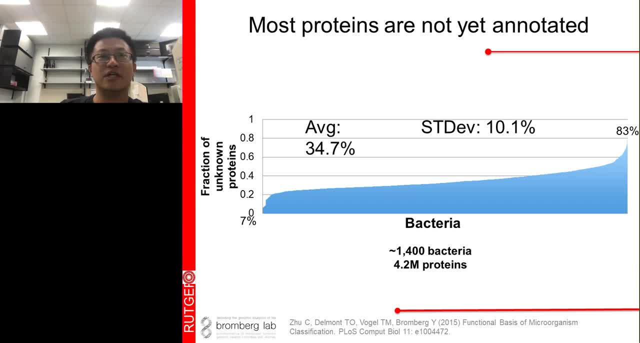 in bacterial genomes are not yet annotated. So here I collected the same 1400 bacteria is of the same data set, which contains 4.2 million proteins. So we can see that on average, about a third of those protein are not annotated. 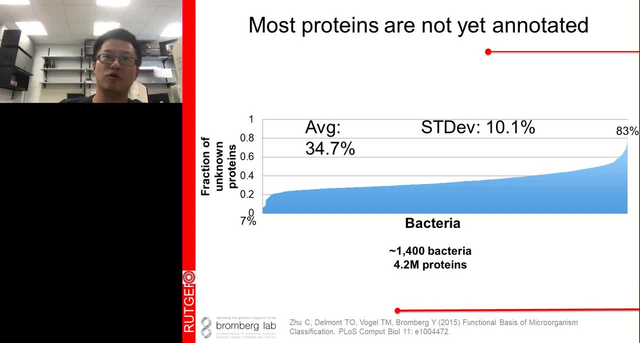 We don't know what the function they perform, And in some organisms, for example the one at the very right, it can be as high as more than 80% of the protein in this bacterium have no annotation at all. We have no clue what they are doing. 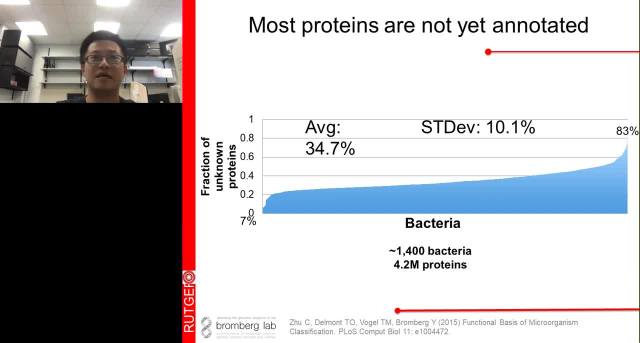 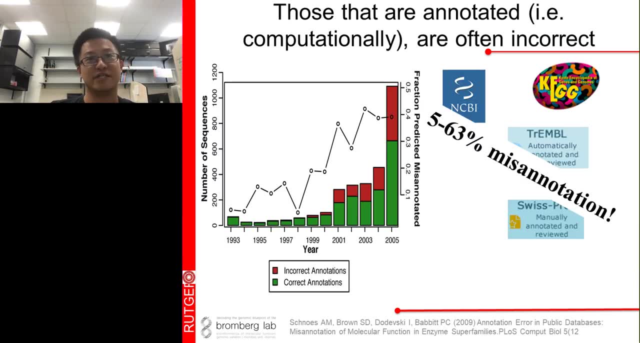 So, yes, no annotation. So, yes, no annotation. So, yes, no annotation is a problem. But then how about those proteins that we do have annotation with? There is also another problem, which is misannotation. So in this paper by Alexander Shnome from 2009,. 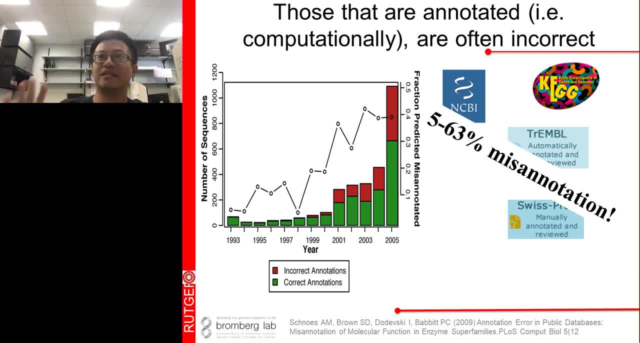 so they have shown that in the big basic public databases like NCBI, CAG or SwissProt there's from 5% to 63% of misannotation In those database And this number is really scary. And it's more scary that once the errors 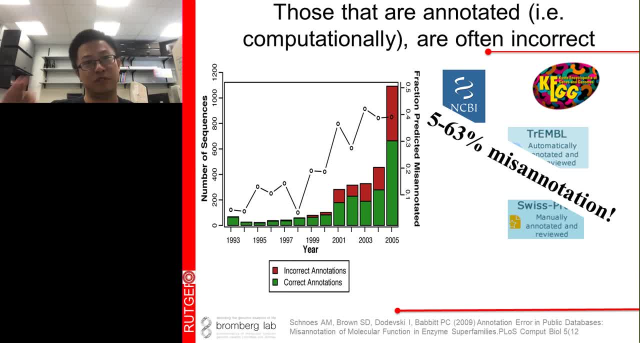 get into this database, they stay there. it's very hard to get them out And these error just propagates to generate more errors, So it just make the situation worse and worse. But then why would we have this misannotation in the first place? 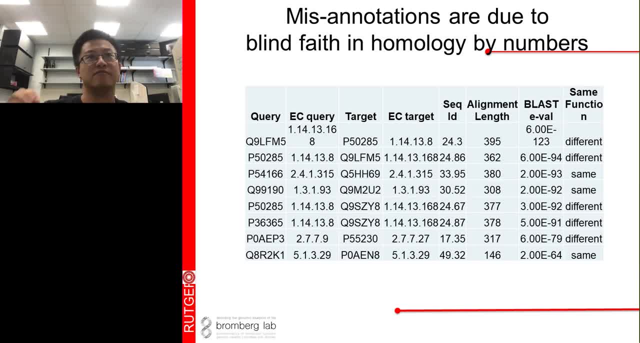 Just to answer this one. So the culprit lies in the blind thing of people in the homology by numbers. So what do I mean by that? So if you have protein sequence with unknown function and they want to figure it out what this protein is doing, 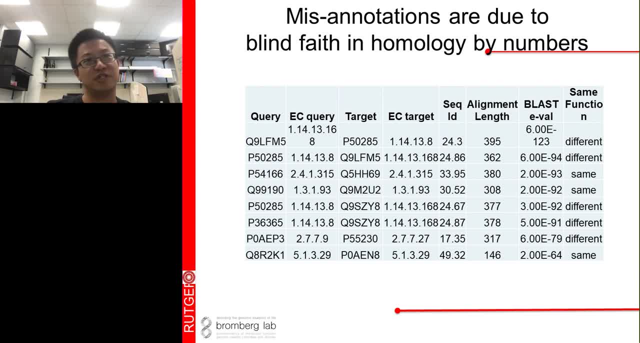 So the most common practice is that you just take it to NCBI and you blast it against some reference database And then you look through the table, look over there. So if you have a protein sequence with an unknown function and you want to figure it out what this protein is doing, So the most common practice is that you just take it to NCBI and you blast it against some reference database And then you look through the database. 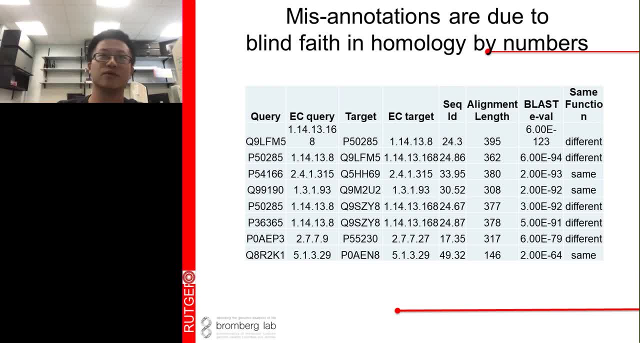 that one Detective evidence through the hits and find out what this protein is doing. So I give you some example here. So if you focus on the first two lines here, so you can see that the blast E value are very decent, which indicating that these proteins. 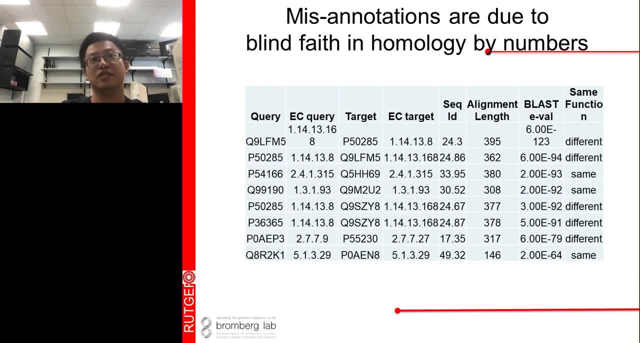 should share the same function. Well, in reality, they're actually not of the same function. So what I'm saying, that there's a function transfer by homology, is not always correct. So is there another way or a more reliable way to measure whether two proteins are of the same function? 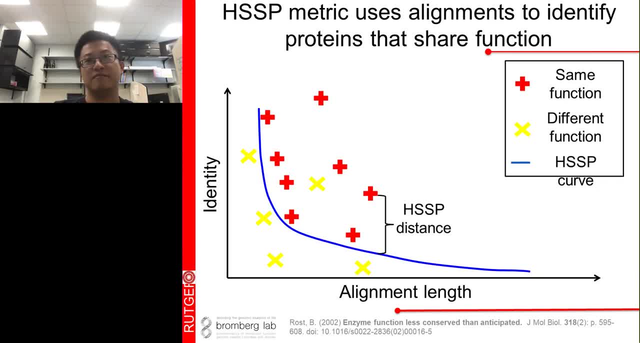 Yes, there is. So this is developed by the advisor of my advisor, which is also who is Dr Brooker Roast in 2002.. He established this so-called HSSP metric. So the idea is that, first of all, 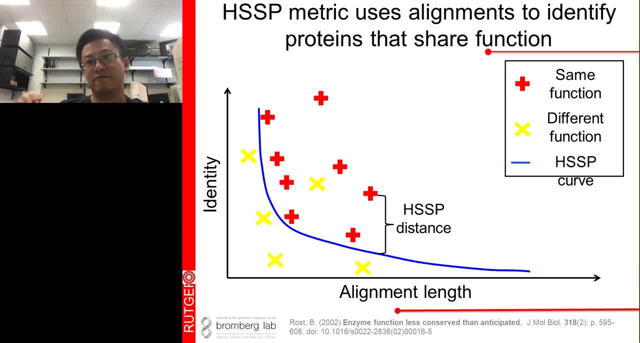 you gather a bunch of proteins from which their function annotation are experimentally verified, which means that they are correct and that we can believe in them, And then you do pairwise alignments for all of them, So you end up with a pair of protein. 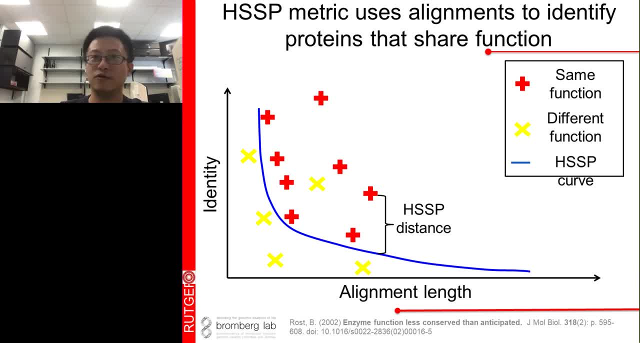 like alignment of proteins of the same function And you also have alignment of proteins with different function, And then you map all of those alignments into this 2D space of alignment length against sequence identity And then you train a curve to separate those same line. 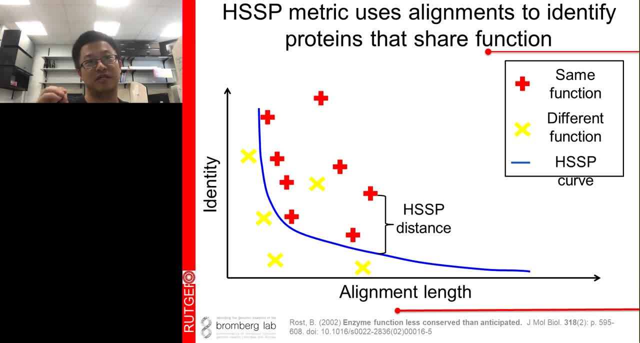 sorry, same function, alignment from the different function alignments, And then once the curve is trained, then the alignment above the curve will be predicted to have the same function And the alignment that beneath the curve will be predicted to have different function. And the distance from the alignment to the curve 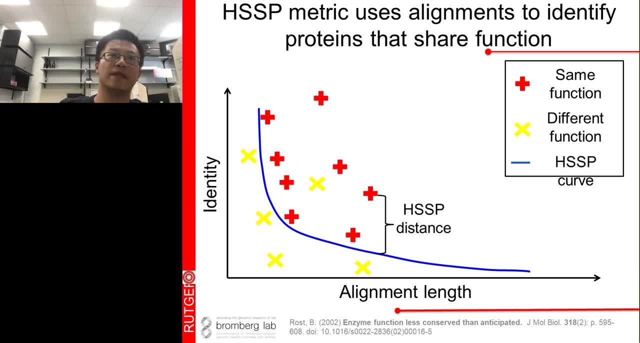 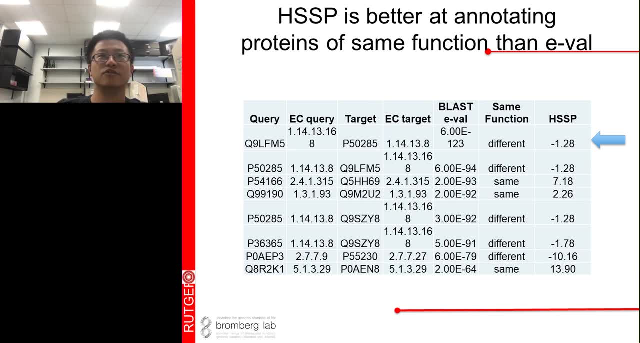 indicating the reliability of such prediction. So now, with this new tool- and let's revisit the example that I just showed you guys- you can see that now, if I calculate the HSSP score of those two pairwise alignment, the HSSP is correctly giving me the information. 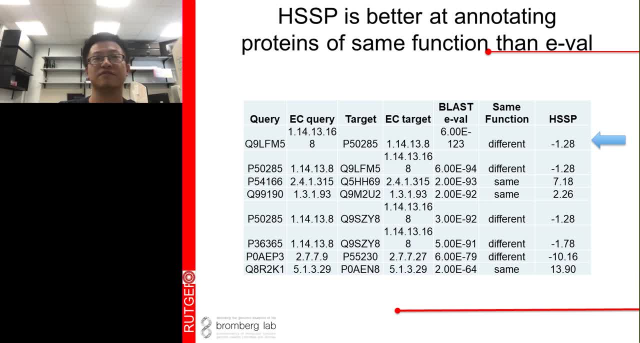 that is a minus value, which indicating that they are of the different function. So the HSSP is more reliable and the HSSP is more reliable, and the HSSP is more reliable and the HSSP is more reliable. 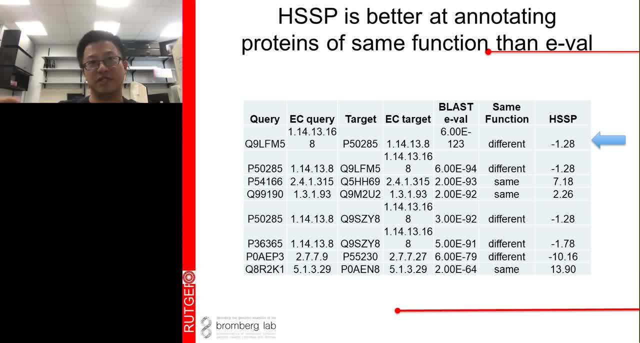 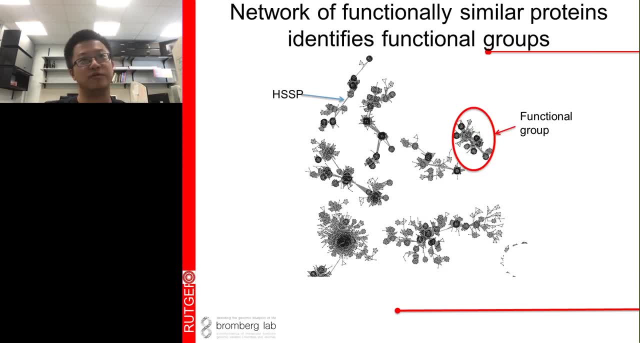 to measure whether two proteins of the same function or not, then blast. So with this tool I was able to actually calculate the HSSP score for all of the pairs in the 4.2 million proteins. And then I put all those 4.2 million proteins. 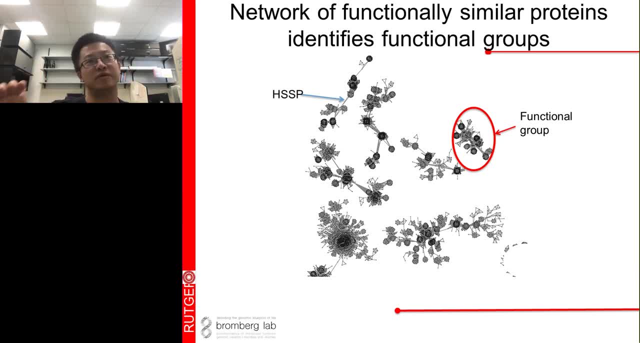 into this big network. So every two protein is connected by their HSSP score. So every two protein is connected by their HSSP score or distance. So in this you can assume that the proteins with the similar function will cluster together. 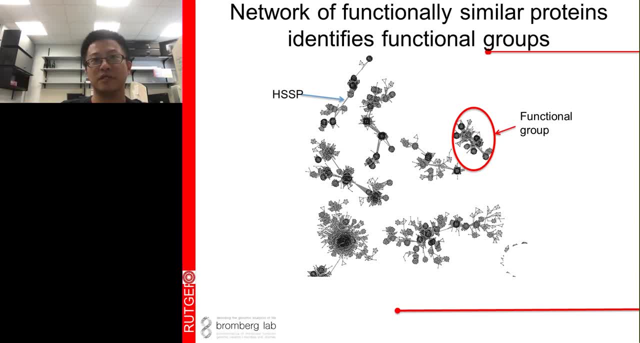 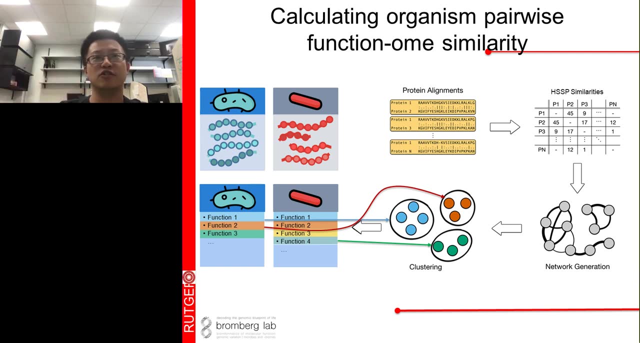 which I can identify later as functional group. The functional group actually just protein clusters that contain protein members sharing the same function, measured by HSSP. So once I have those. so this is a flow chart of the whole procedure. So once I have those, 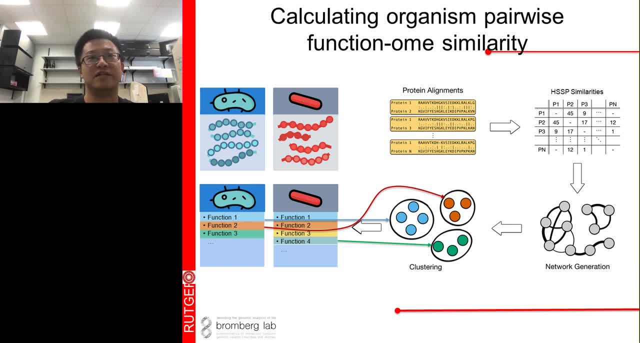 so this is a flow chart of the whole procedure. So once I have identified those protein clusters, what I can do is that I can map each bacteria to a list of molecular functions that its genome contains. So, for example, both the blue and the red bug has function one. 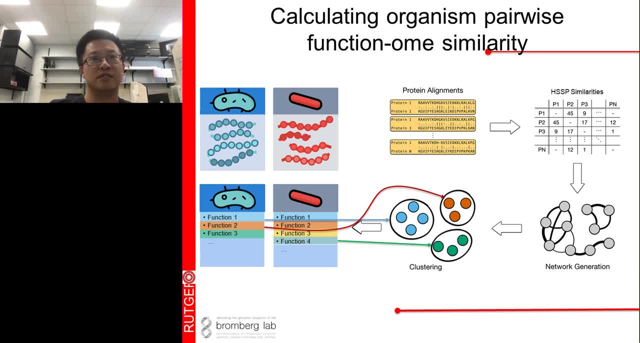 and the function two And the function four is unique to the red bug And the function four is unique to the red bug. So with this I can further calculate the functional similarity between every pair of proteins, between every pair of proteins, By just comparing the similarity. 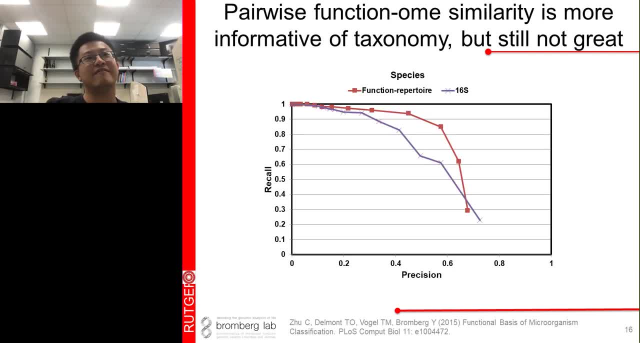 between these function vectors. So if I use that similarity as a new metric to identify if two bacteria of the same species or not, here you can see a significant and obvious performance scan comparing to using 60S RNA. But, however, it's still not great. 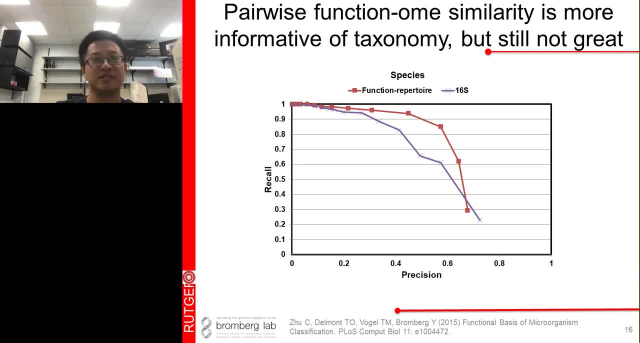 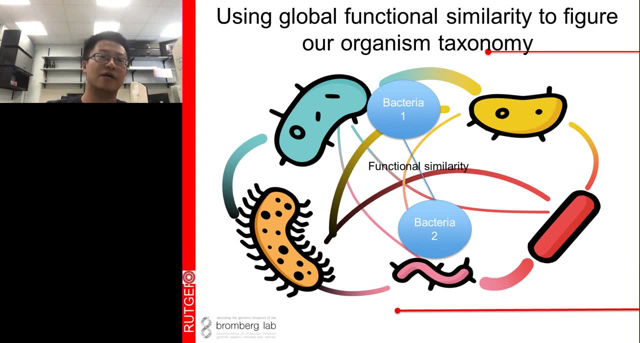 because you can still only retrieve like around 70% of precision. So then what right? So we take the idea of like all right, if the pairwise alignment or the pairwise comparison of bacteria does not really work, then let's try the network. 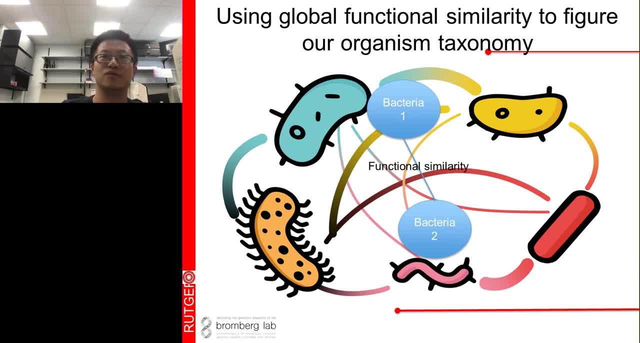 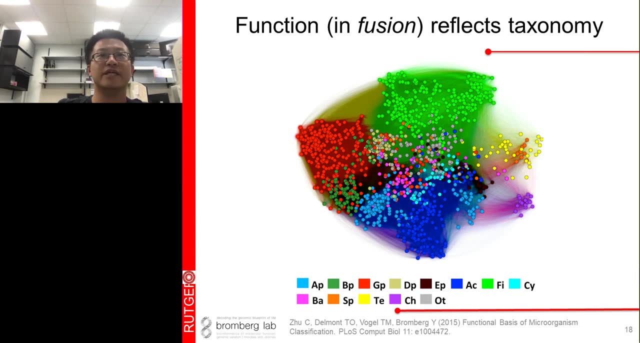 So now we can actually put all of the bacteria into a big network and connect them by the functional similarity. In the same notion, the bacteria that are functionally more similar tend to cluster together as well. So if I do this to all the 1400 bacteria in my data set, 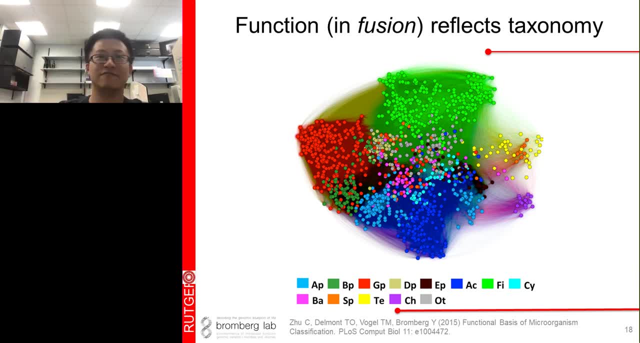 we get a network somewhat like this: like a fish, It's a fish network. So here in this layout of the network, all the organism nodes are colored by the phyla and the major classes. So we can compare this organism clustering to the taxonomy. 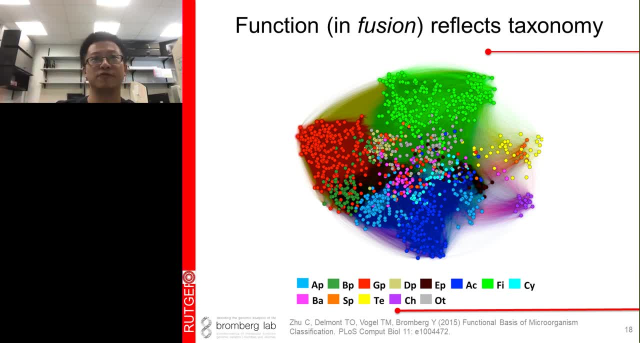 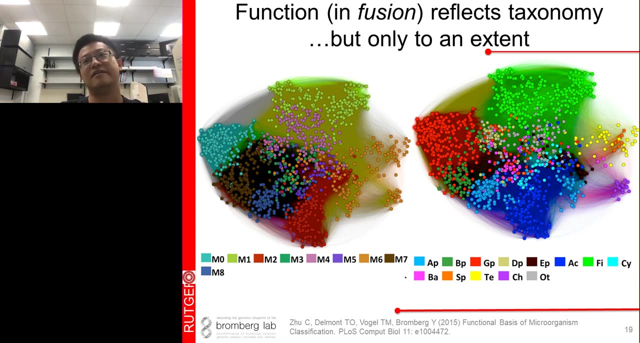 And we can see that this network, which we call fusion- So there's a fusion network- actually reflects taxonomy, But, however, only to an extent, because here, if I were to use computational methods to identify these explicit and the strong sub network, 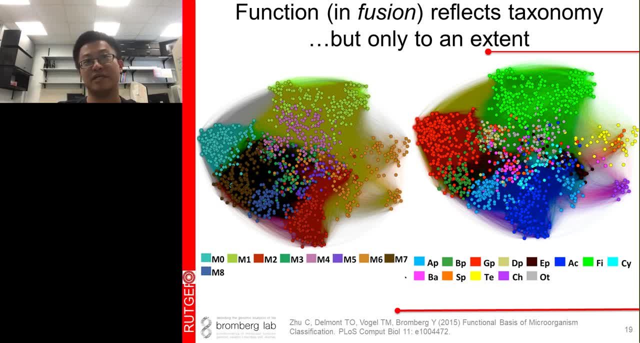 within this fusion network. by saying sub network, I mean that the sub network have very strong within network connections and the very weak across, I'm sorry, have very strong within sub network connections and the very weak across sub network connections. 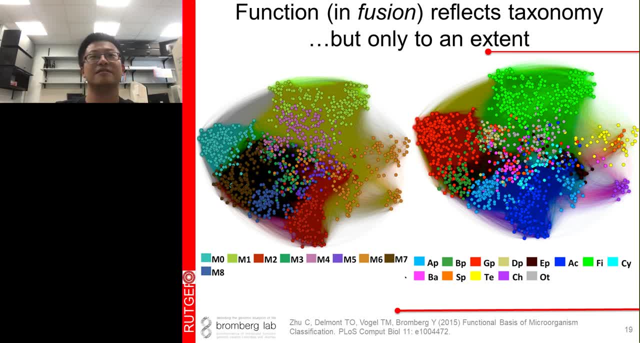 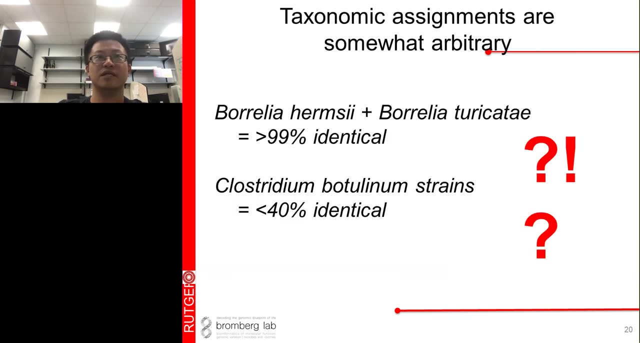 So if I were to identify these sub networks and we can see that they do not entirely overlap with the current taxonomy, So why is that? The sub network is totally driven by the function similarity But the current taxonomy is not, because it is somewhat. 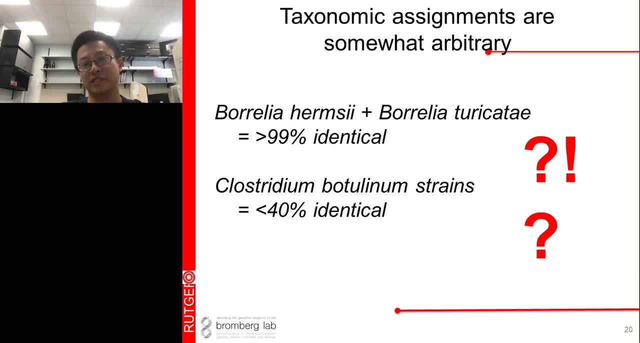 arbitrary, like what I mentioned in the beginning, by Darwin. So I give you an example here. So at the top, these two Borrelia species: they are functionally more than 99% identical But however, they cause different subtype of diseases. 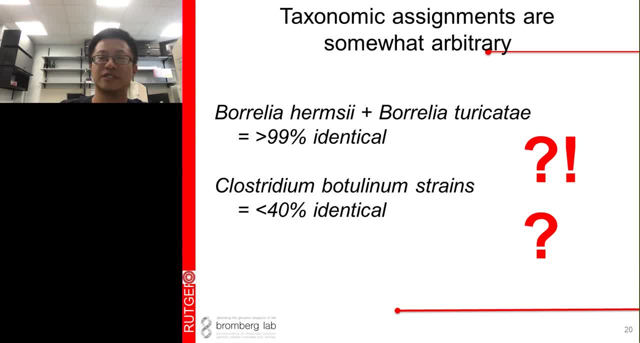 And we just decided to put them into different species And at the bottom this Clostridium botulinum strains. So they are functionally very different, less than 40% identical from one another, But, however, because they all cause the same type of disease. 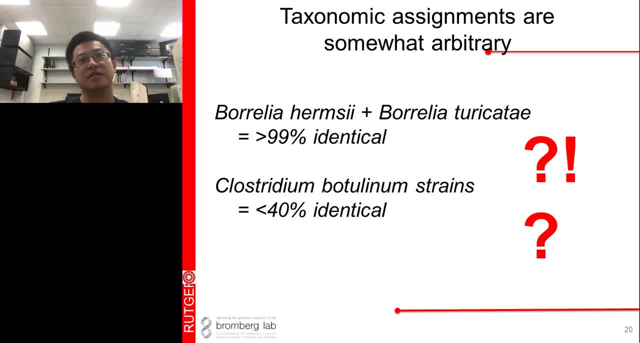 we put them just in the same being in the taxonomy. So this is very arbitrary, just like the bird example. unless you're an expert that spend your life studying these specific bacteria, you will not be able to know what is going on. 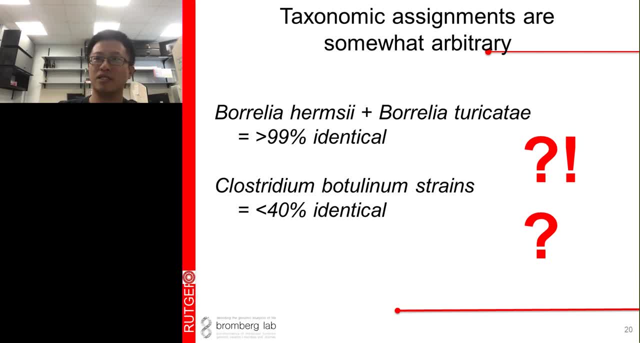 And this is actually also almost impossible, and this is actually also almost impossible- made it almost impossible to process, like in this large scale computational analysis. So I will leave an open question here. So do you think the current taxonomy needs some modification? 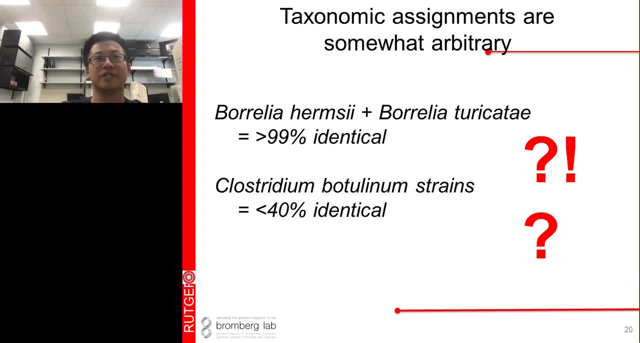 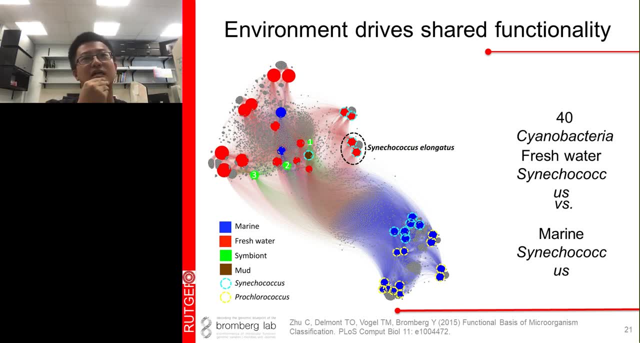 How would you address this? like contradiction here? I would be happy to hear your thoughts. So here I'll give you another example showing, like all right so, how function is affected by the environment. So these are: this is a network of 40 cyanobacteria. 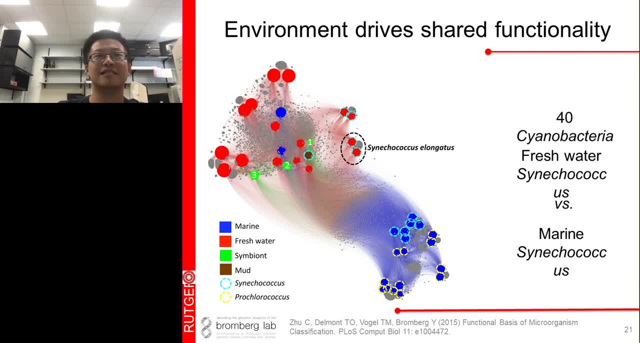 And I want you to focus on the nodes with the cyan ring. Those are the synecococcus, which is a genus of the cyanobacteria. So you can see that those marine synecococcus are functionally very different from the freshwater synecococcus. 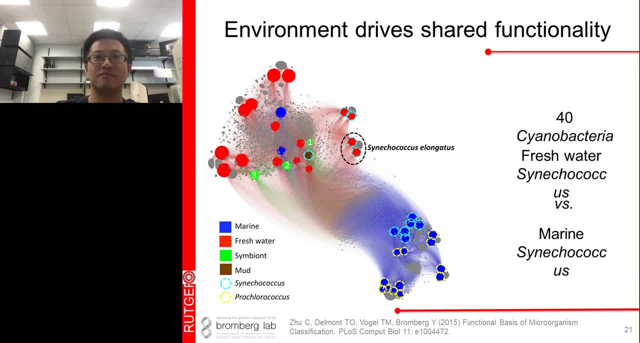 And they are actually functionally very different, very similar to another marine cyanobacteria, which is the Prochlorococcus. Those are the ones, the nodes with the yellow ring. So here we see a clear signal of how microbial function is driven by environment. 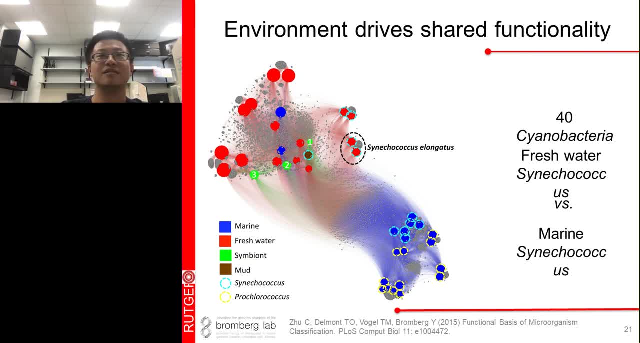 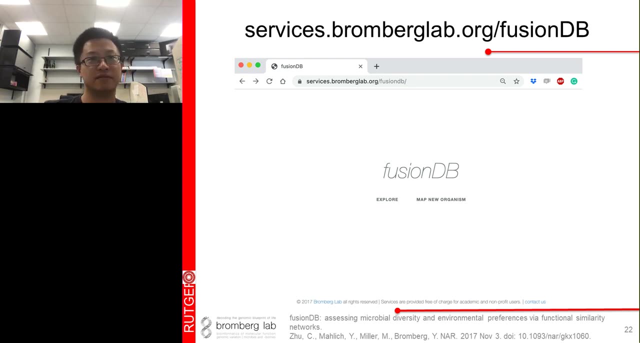 And the current taxonomy is not seen, cannot see this change or this difference. So, in order to make usage of our data, we build FusionDB, which is the online database which stores all of those 1400 bacteria information that we calculated, function and environment information. 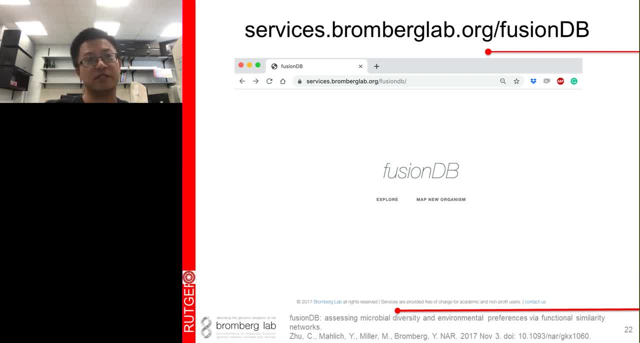 So in FusionDB we allow you actually to submit your organism of interest, submit genome to us, And then what we will do is that we're gonna map it to the Fusion data. So once the mapping is done, you're gonna see a result page. 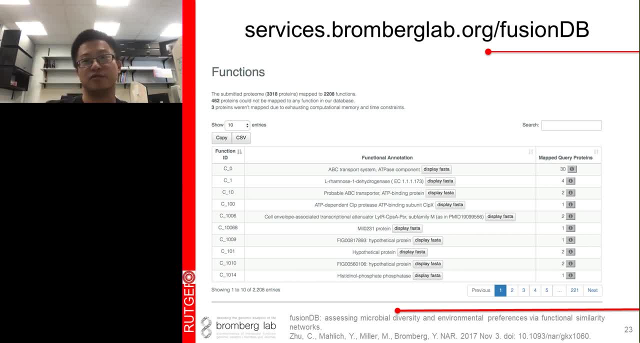 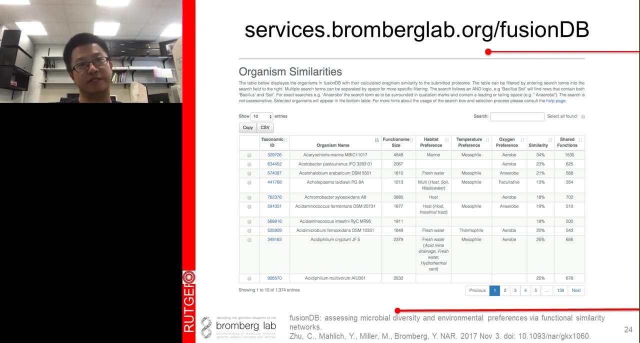 like this. So first your organism will be mapped to all the molecular functions that we defined. So remember those protein clusters in the big network. So we're gonna first map your organisms into the list of functions And then we will calculate for the functional similarity. 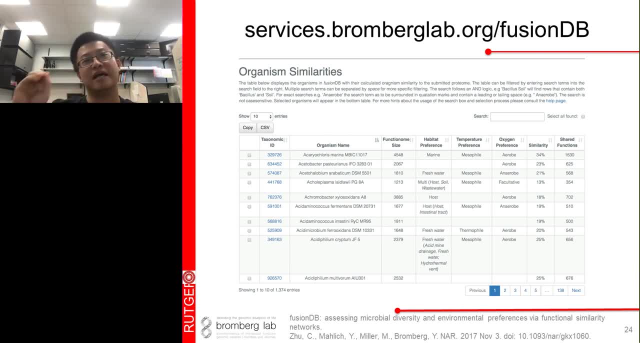 between your query organism against every single reference organism in our database And also, as you can see here in this picture, each reference organism is associated with environmental metadata which includes like temperature, oxygen and habitat. So you can further select the organism of your interest. 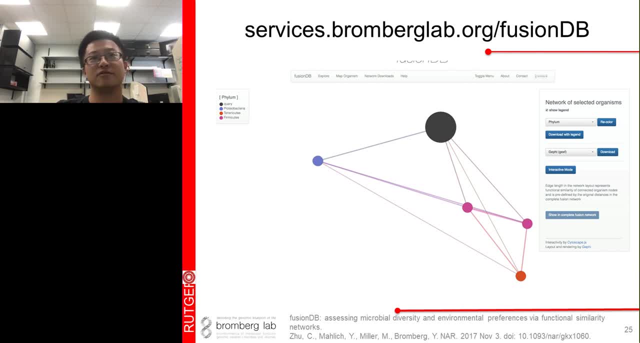 and using those and your query organism together to create these network realizations on our database And you can color them by taxonomy, by environment data, to try to find the patterns and why, to find out what is the reason to cause this function, similarity between these organisms. 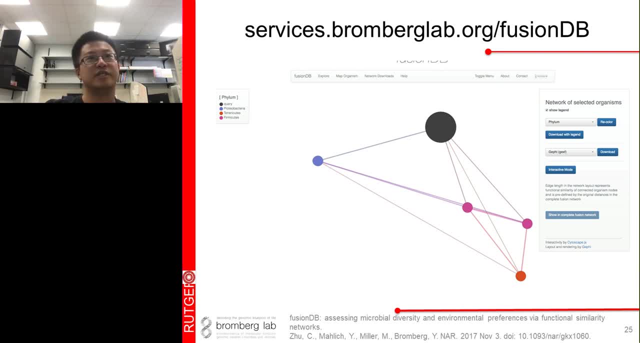 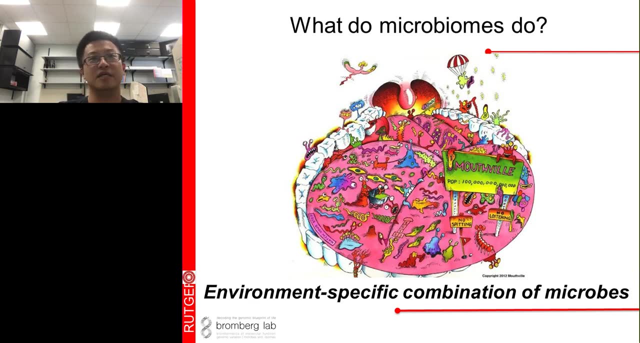 So that is so much of the genome functional annotation And I will be moving on to the microbiome. So basically, microbiome is just a community of bacteria that live in certain environments. So instead of looking at the one bug now, we're looking at 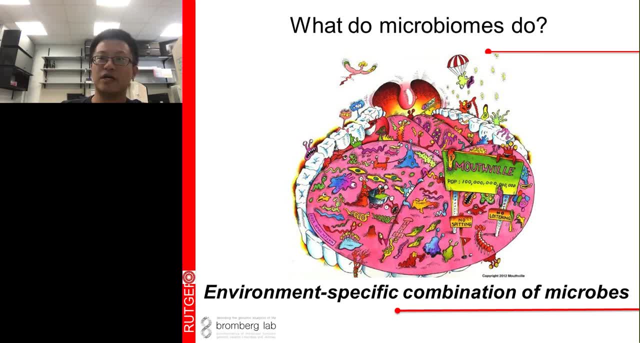 a group of bugs, So there are multiple ways to study them, but one of the most commonly used one is using metagenome, which is a sequence- all of the genetic material from all of the bugs in this environment, And after that we get these short DNA fragments. 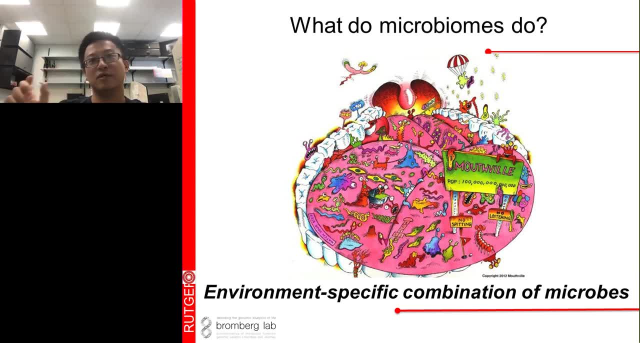 which we call reads. So there is one way to assemble the reads into Contig and reconstruct the whole genome. So I'm not gonna talk about those, I'm gonna talk about the function annotation which is a way to do that. but I'm gonna talk about the function annotation. 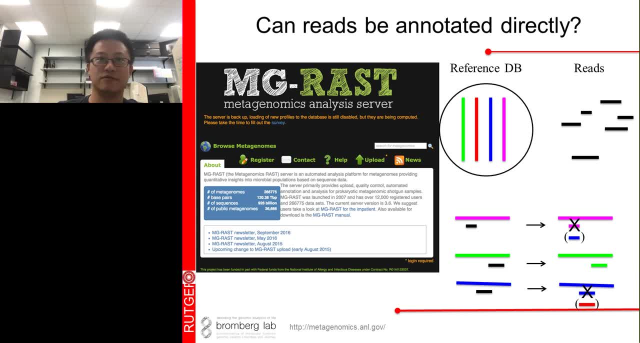 which is one of the most commonly used ones. So just to give you a little bit of an example, today I'll be talking about directly annotate function from the reads. So there are already some resources dedicated to that. For example, MG-REST is quite a famous one. 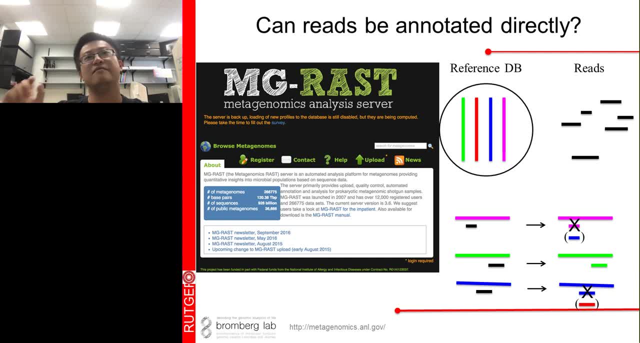 So it annotates the function directly from the reads. So how it does it that? So how does it do it? reference proteins And then, if it matches, then the function of the reference protein is transferred to these reads. But the problem with that is because these 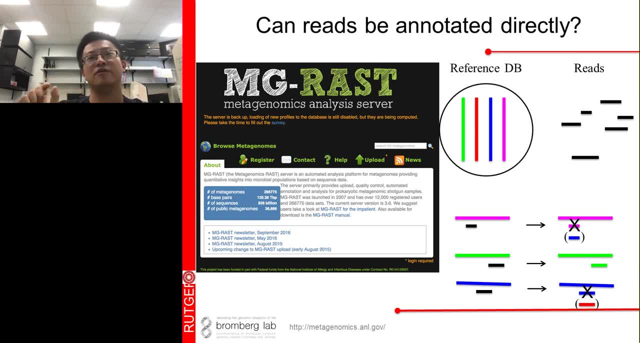 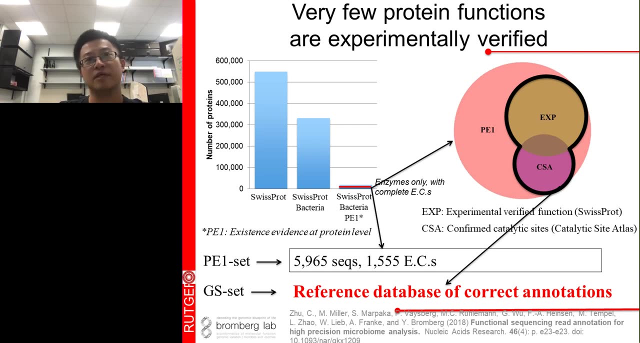 are super short alignments. Therefore you have a lot of unspecific binding, which means that you end up with a lot of false positives. And another problem is, again, as I mentioned before, the annotation quality of the reference database is questionable. 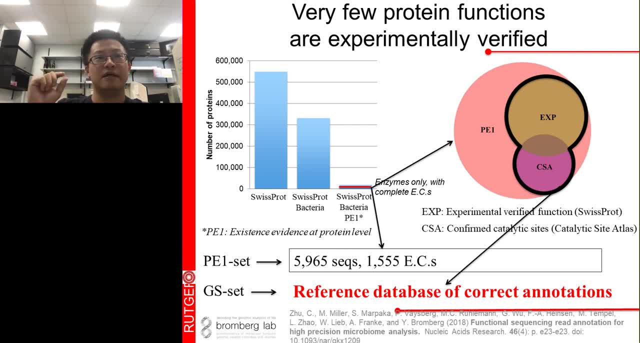 So here you can see that the number. so here in this chart, the bar on the very left, is the overall number of proteins in SwissProt. So SwissProt contains only manually curated proteins, Manually curated with. proteins with functions are manually curated. 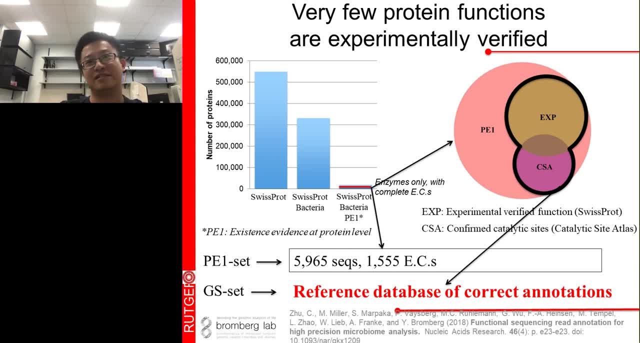 And then, among all of those, how many proteins that we actually have generated and see it in lab? There is only less than 6,000 proteins that we have seen it in lab. So that is the existence evidence at the protein level. 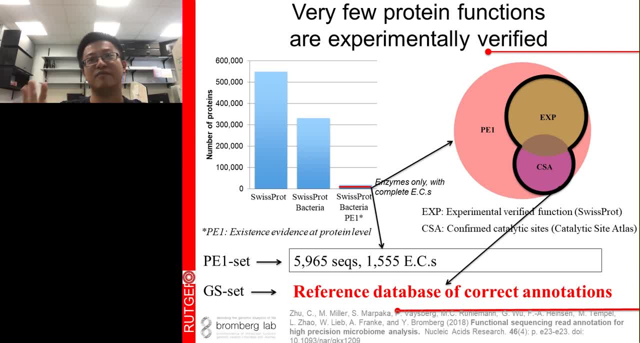 So out of half a million- around half a million- of the manually curated proteins, only 6,000 proteins. we have actually seen the protein. The other ones we only know the sequence. We have never seen the protein itself. And among these 6,000 proteins there are actually: 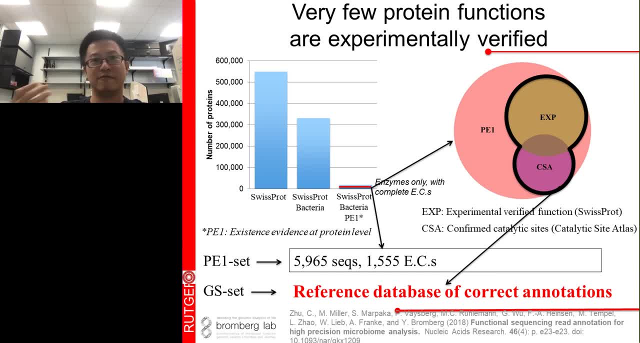 even a smaller fraction, which is fewer than 3,000.. So that's a lot, So that's a lot, And that is good excellence in such an important function. And so you see, there are almost 50 to 100,000 protein sequences. 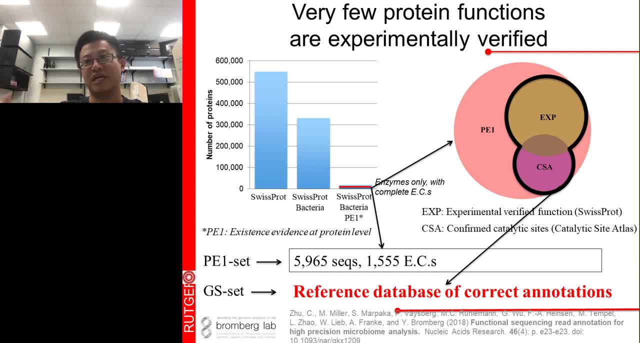 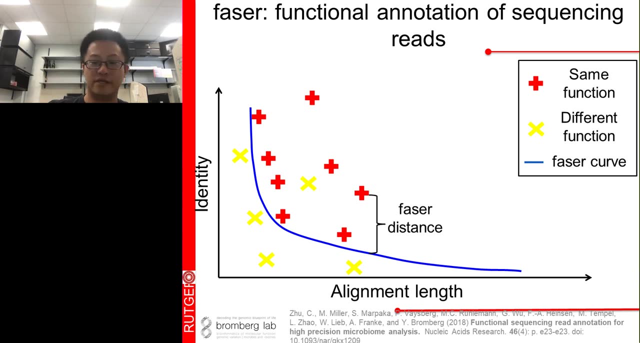 whose functions are actually experimentally verified. So we are talking about a very tiny core set here that we have a high confidence in their functional annotation. So we use this set and what we do is that we use the same idea to train a curve. 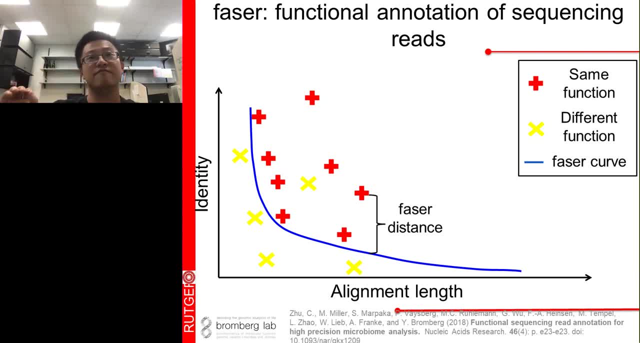 to separate alignment, But however, here the same function are the func-. I'm sorry Now, but however, here the alignments are not protein-protein alignment anymore, But the short reads align to the full length proteins And once we train the curve that separates. 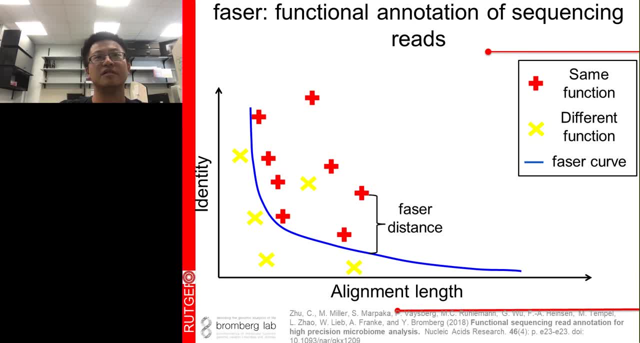 those same function alignments from the different function alignments. same idea. We can calculate this Now. we call this new metric phasor. We can calculate the phasor distance, which indicates the reliability of the function predictions as well. So we compare the phasor to CyBlast. 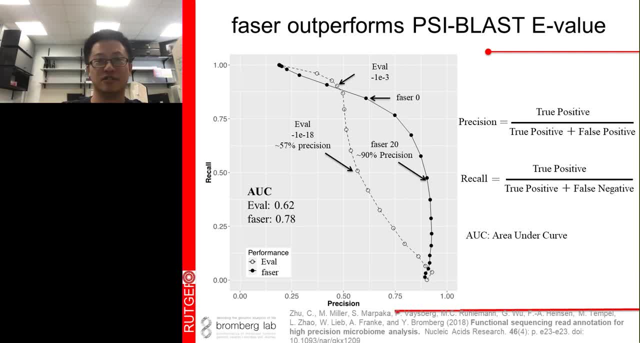 in terms of the performance, like: how well can we annotate functions So we can see that the phasor outperforms CyBlast E-value by a lot? With phasor you can actually reach around 90% precision, which is amazing in terms of annotating the short reads. 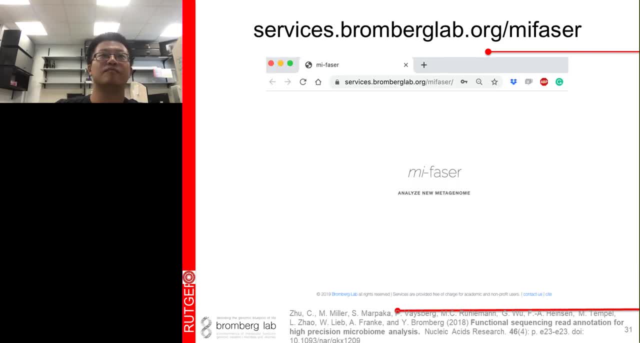 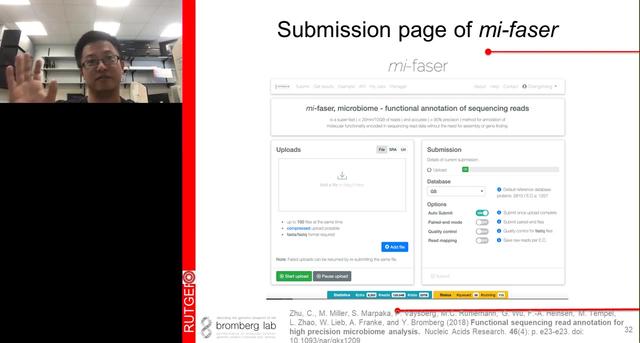 and the long reads, And we also created an online service which is called My Phasor, which is available at the website here. So in My Phasor, we accept your submission of your metagenomes And we will annotate it for you using the phasor algorithm. 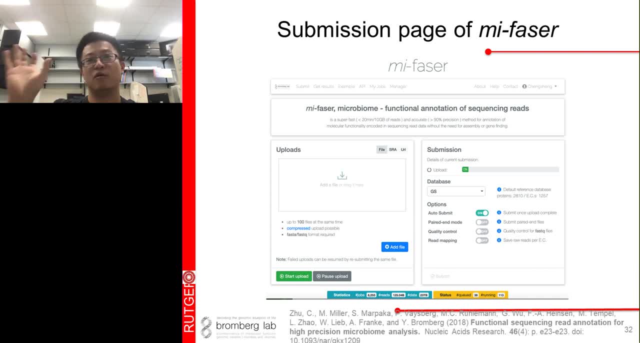 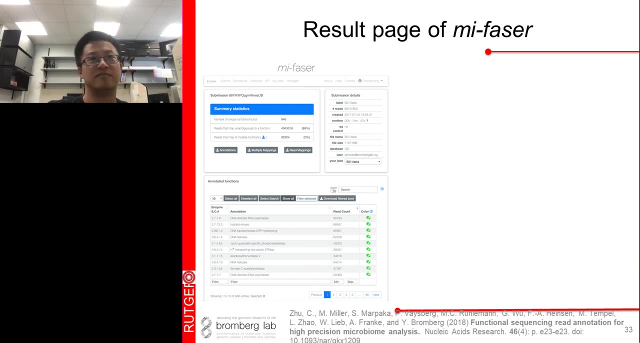 against that gold standard database where every single protein is functional. annotation is experimentally verified. So once your job is processed, the result looks something like this. So on the top page there are some statistics and descriptions of the job And the bottom is the read abundance table. 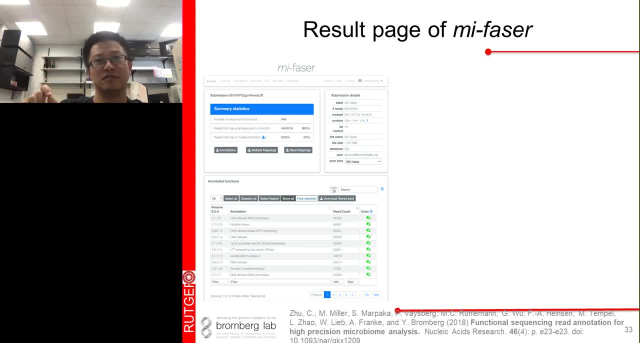 So you have: each line indicates one function. So here all the functions are reliable because they are experimentally verified. And then you have the number of reads that map to this function. So the idea is, with my phasor I can turn your metagenomes into functional profiles. 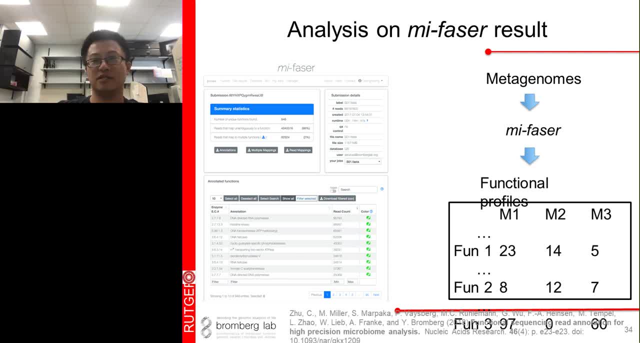 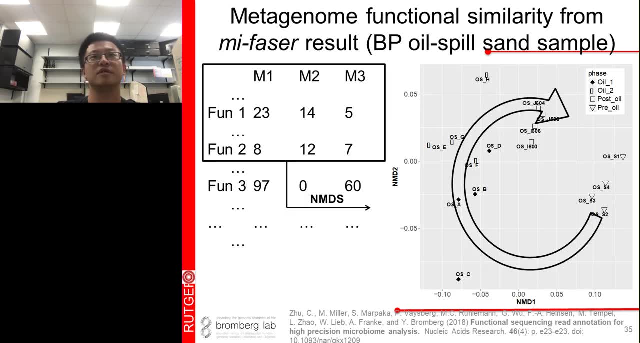 Looks like this And from there we can do actually a lot of different analysis. So I'm going to give you some examples of what we have done on different samples. The first one I want to show you here is actually based on the BP oil spill sand data. 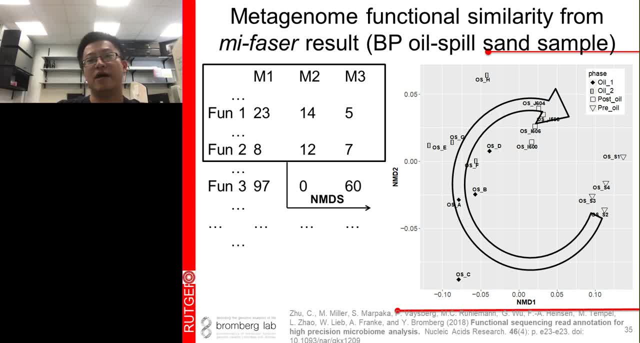 So I'm sure you heard about this. It's very nasty. But however, for this group they actually had the sand data before oil, during the oil phase, and then have the sand sample after the oil has been degraded, so the post-oil phase. 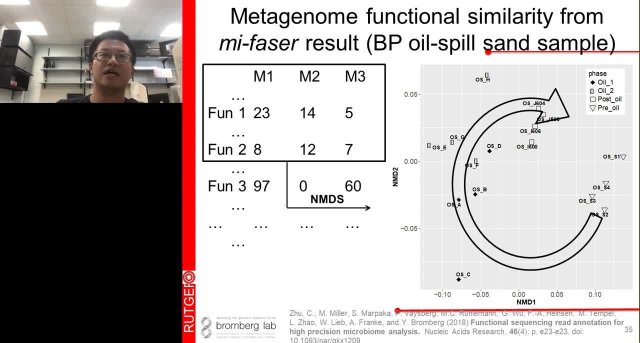 So we analyzed this data set with my phasor and then used MDS, which is a visualization method, to compare the functional similarity between these metagenomes in the data set. So you can see it's actually pretty Well separated between different phases. 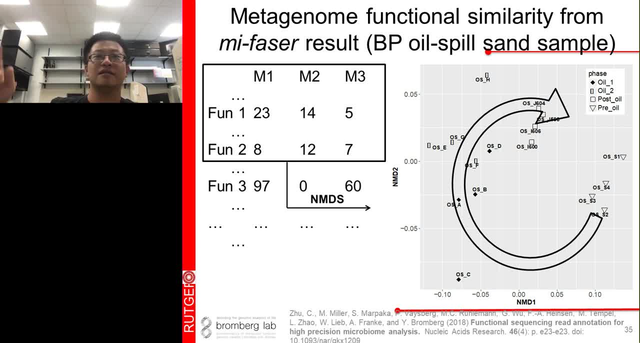 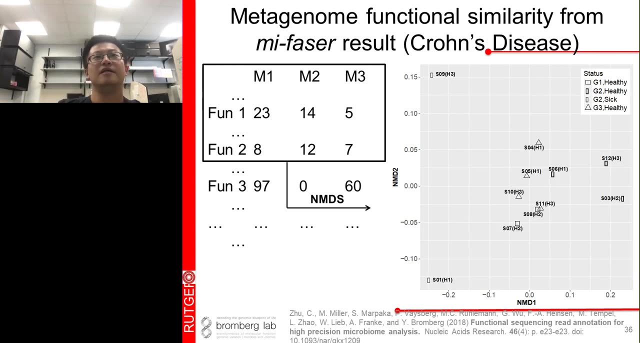 But what is more interesting here is actually you can see that this, from the pre-oil to oil phase and then to post-oil phase, is kind of showing the sand microbial community is recovering from this contamination. And another example I'm showing you here are human data. 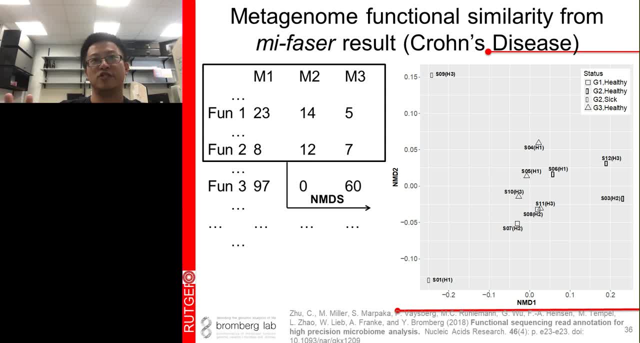 So, which is there are two patients with Crohn's disease and they're healthy. They're healthy relatives. So what you can see here is that for these two patients, so we have their gut microbiome samples, So their gut microbiome are actually 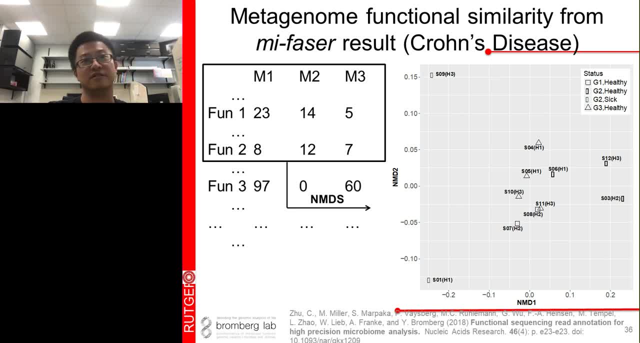 functionally very different from their healthy relatives. And which is more interesting is that even between these two patients their gut microbiome functions are also very different. which indicate the possible. which indicate the possible different mechanism of the Crohn's disease. 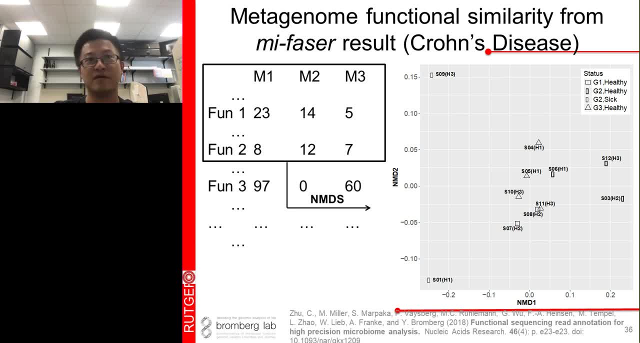 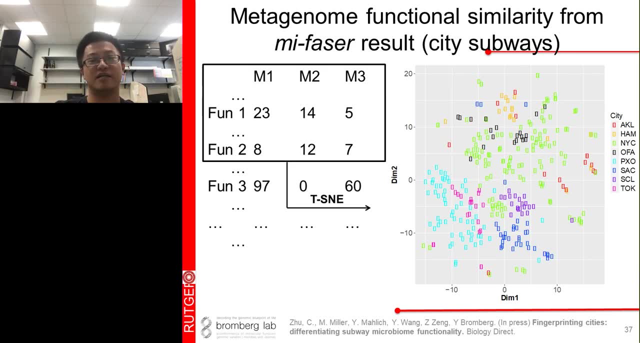 pathogenicity or how that reacts with that microbiome, so on, And this is also oh sorry. So this is also done by NMDS. So, from our experience, NMDS, this visualization method is very good for small sample size. 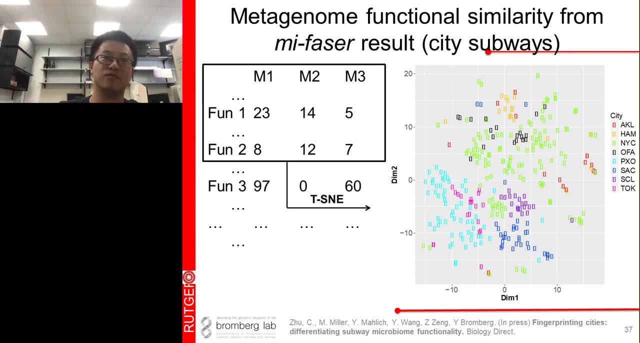 But, however, for big sample size, like a tisany embedding, is more suitable. So what I'm showing you here, the last example- is that these are from the city subways. The microbiomes are sampled from the city subways from various cities from the world.